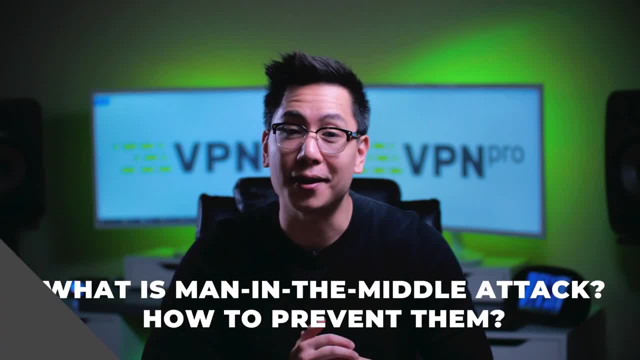 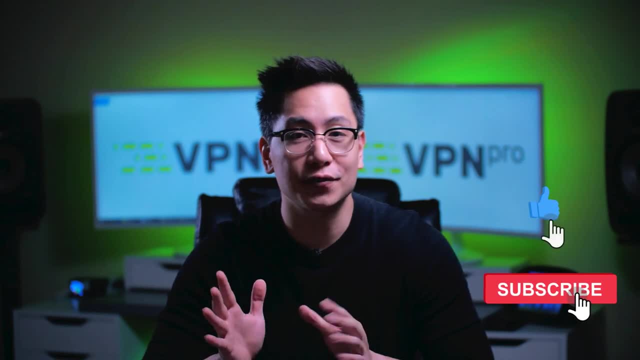 you everything about man-in-the-middle attacks and how to prevent them. But first, before you fall victim to any unsolicited attacks or if you want to enjoy promotions and discounts, make sure you subscribe to our channels for the latest and all the best VPNs. You might use public Wi-Fi networks often, and why. 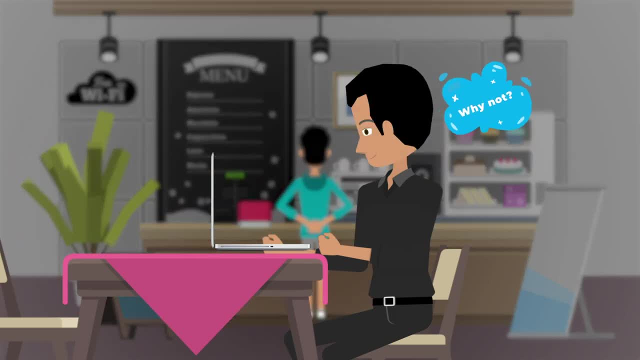 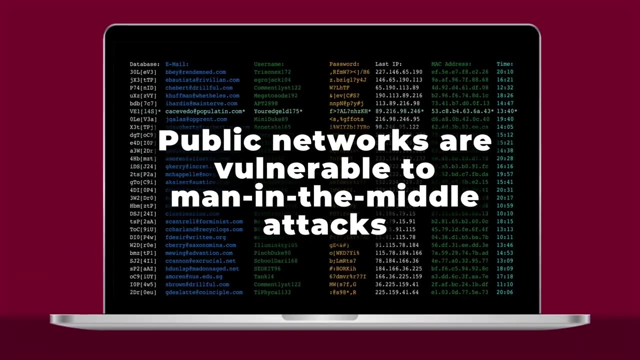 not. It's totally free and a convenient way to not spend your mobile data, But have you ever thought about your internet and device security when doing so? Many of these public networks are susceptible to man-in-the-middle attacks, where your data can be read, stolen and altered by cyber criminals Man-in-the-. 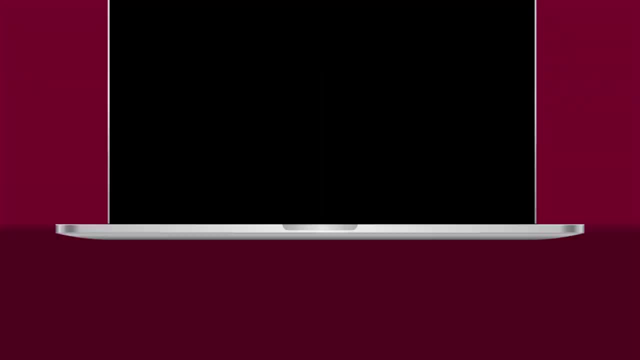 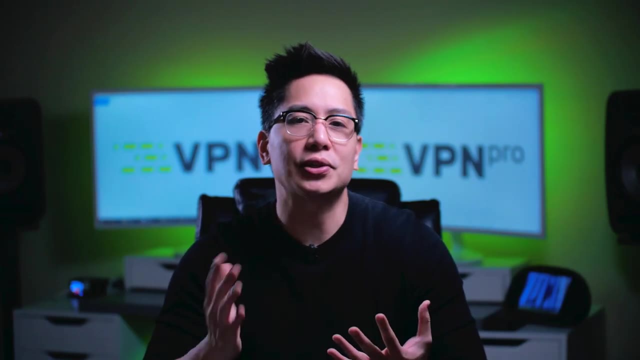 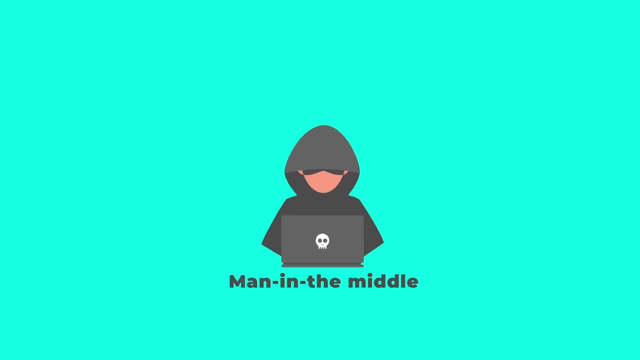 middle attacks are some of the most common cyber attacks. Why? Because it's easy and potentially very lucrative. Not only can you expose your financial details this way, but you're also resclusing all your personal valuable information because of it. So what are man-in-the-middle attacks? As the name suggests, the bad guy. 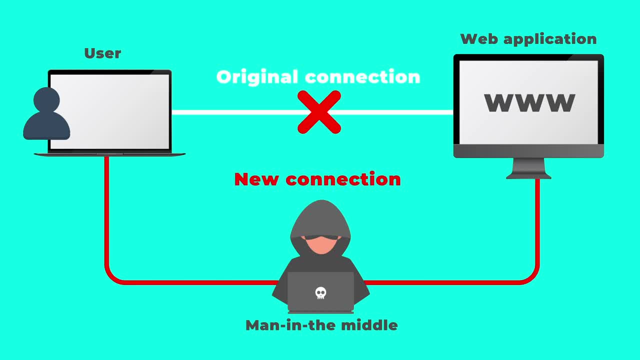 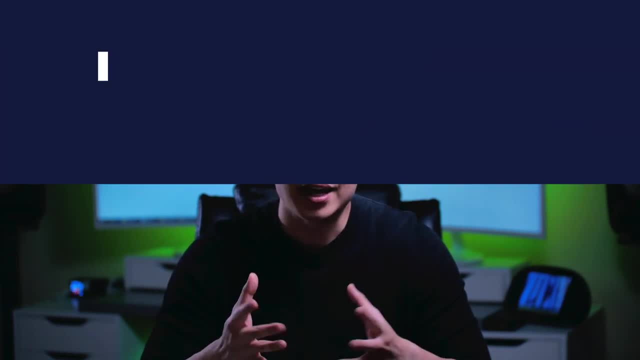 inserts him or herself on a communication between two devices and reads the traffic without anyone noticing. Usually, those two devices are your laptop and the Wi-Fi router. If you're not using an encrypted connection, which usually happens when you visit an insecure website, the man-in-the-middle 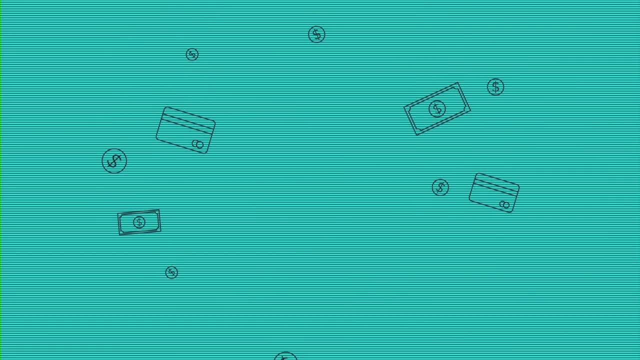 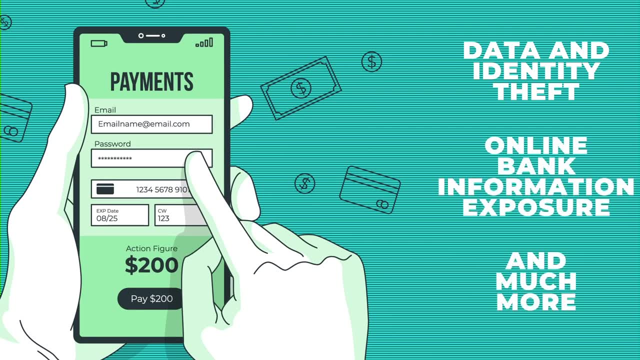 can learn all sorts of sensitive information. So, in short, a man-in-the-middle attack can lead to data and identity theft, online bank information exposure and any other kind of security threats. So what are man-in-the-middle attacks? The first thing to keep in mind is that you're not the only one who is 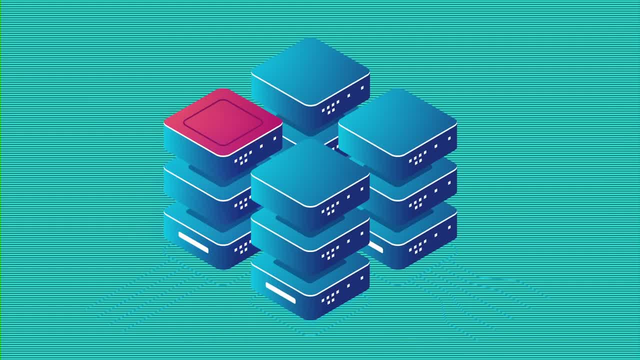 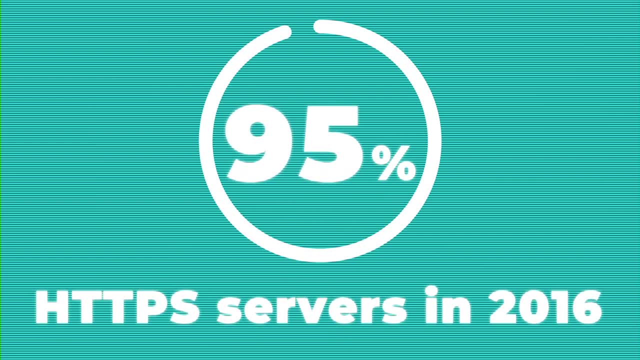 vulnerable to man-in-the-middle attacks. Even HTTPS servers are very vulnerable to man-in-the-middle attacks. As recently as 2016, it was found that 95 percent of HTTPS servers are vulnerable. Scary right, It's not just about laptops either. I. mean, think about it. What device do you use the most and need the most protection on? That's right, your phone. You carry it with you to the shop, to the cafe, and you even connect the strange public Wi-Fi connection so you don't have to use your mobile data. 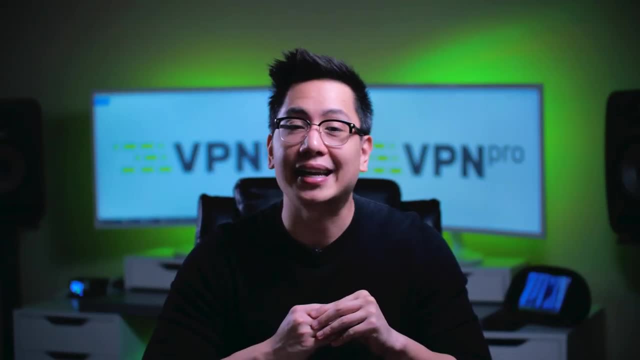 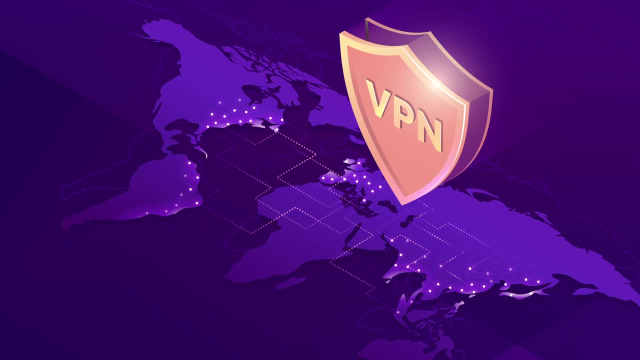 Believe it or not, phones are just as susceptible to man-in-the-middle attacks as any other device. Fortunately, there are ways to preventing man-in-the-middle attacks, and VPN providers are the best way to go. These services encrypt your connection, which will protect you from man-in-the-middle attacks. 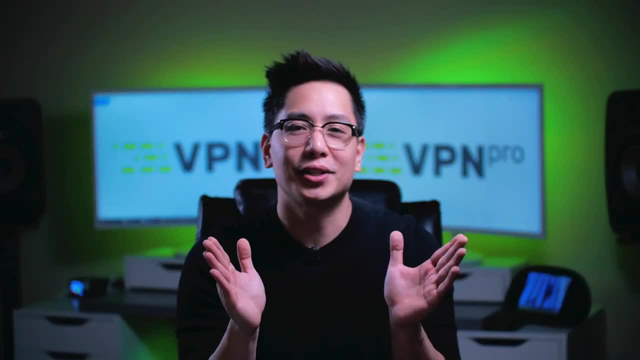 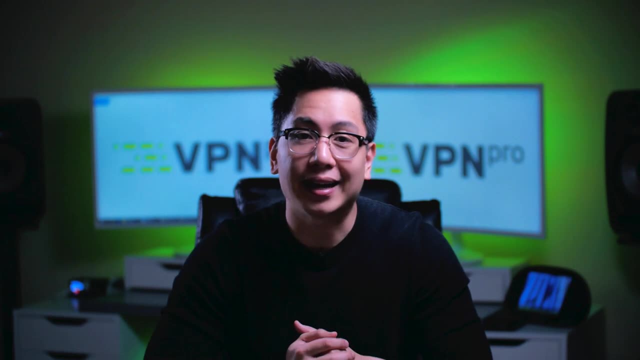 even if you're visiting insecure HTTP websites. Be sure to click the pop-up banner to see our full list of the best VPNs and get up to 84% off. If you're not sure which VPNs are the best, I can tell you now that you should either go.